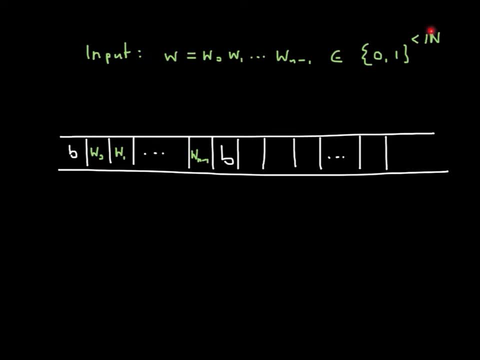 a string w given over the binary alphabet And this, as defined in the last lecture, will be put on the worktape and each bit of the input in one cell Initially. there are no other non-blank cells on the tape. so to the left and the right of 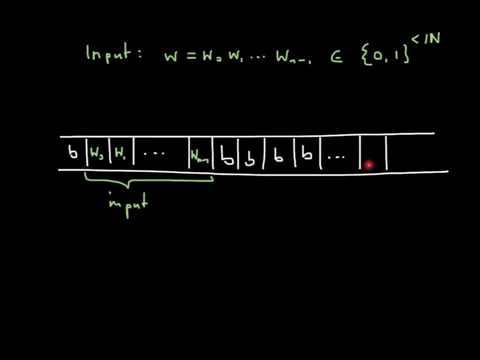 the input are only blank cells. But assume now our input is of the form that we want to recognize. So assume we have 0, 0, 0, 0, and then 1, 1, 1 in the input. 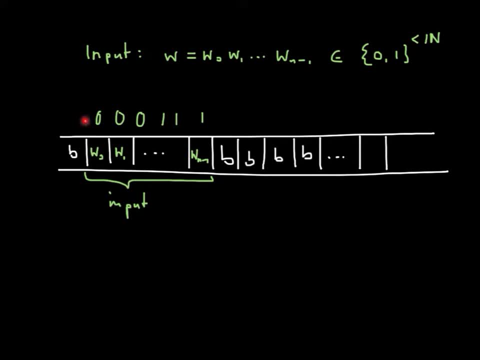 The idea now would be to scan the input from left to right. Remember we always start on the cell that is to the left of the input. Scan it from left to right And first, whenever we read 0 here, use an area to the right of the input, over here. 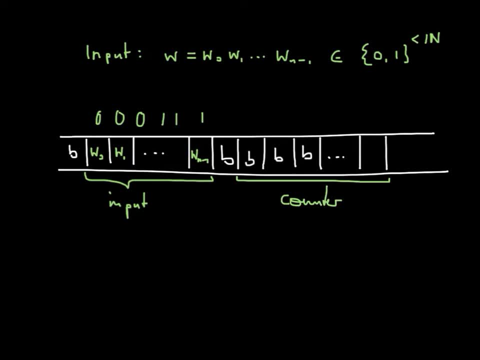 as kind of a counter area, where we create a counter that counts increases whenever we read a 0. So we increase this counter by 1.. And then, when we stop reading 0s and read 1s, we decrease the counter here accordingly by 1.. 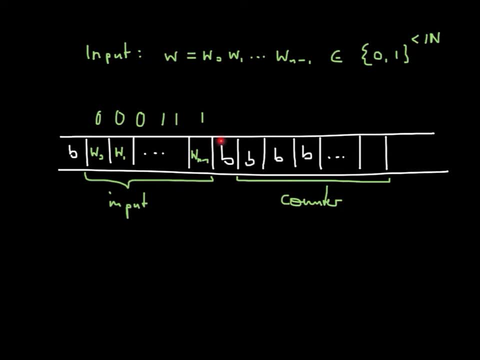 And then at the end, once we hit the blank here, that means we have read through all the input. we'll just check whether our counter in this area here is also back to 0, or blank, or if there's still a symbol left there. 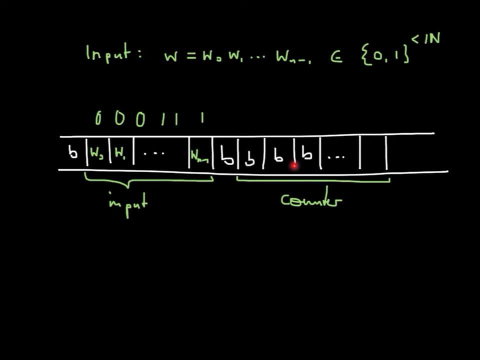 And then we can decide accordingly. So again, the idea would be scan the input from left to right. As long as we read 0s, increase the counter. decrease the counter once we read 1s, by 1, accordingly, Once we hit the end of the input. 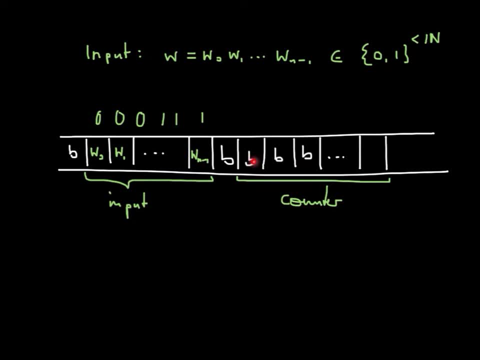 we check the counter whether it's all the way back to 0.. We have to be a little bit careful, though, when devising our program. Namely, we could have the situation where we have the same number of 0s and the same number of 1s. 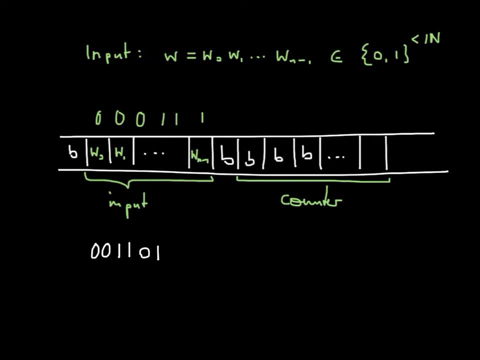 in the input something like this: So if we just went through the input now from left to right and increased the counter every time we read a 0 and decrease every time we read a 1, this input would also result in a counter 0.. 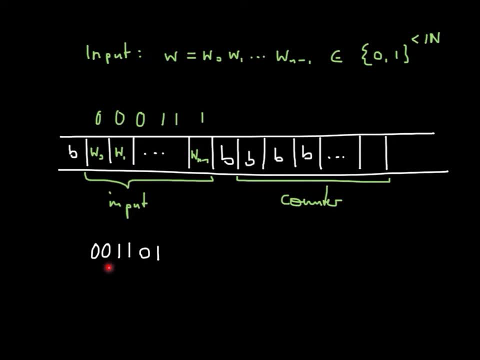 But of course it is not of the form that we want, So it's not of the form. 0 to the n, 1 to the n. So once we read the first 1, we have to account for that in our program by saying: OK now. 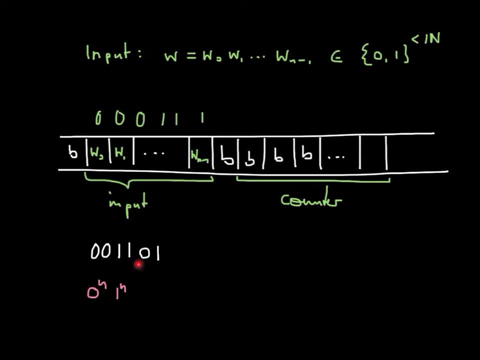 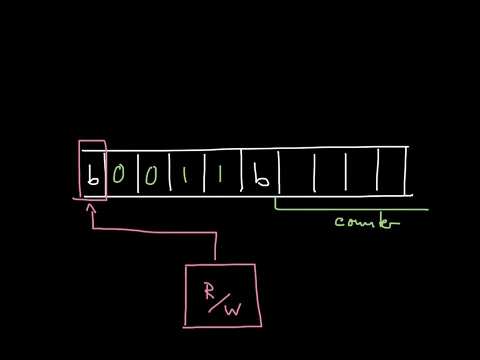 from now on. we don't want to read any more 0s, Otherwise we'll output 0 that is not accepted right away. So let's try to work out the instruction we need for this machine in a little bit more detail. 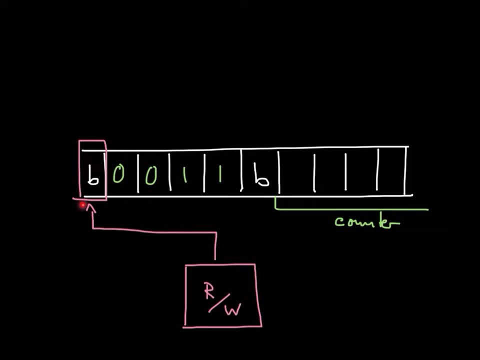 So, as usual, we start by pointing the ReadRightHead at the cell immediately to the left of the input. And now, in the first step, we would just go to the right to start reading the input. So we moved our ReadRightHead just one to the position. 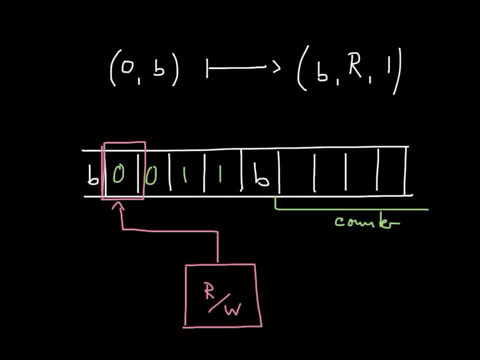 to the right In terms of a transition function or instruction. this would look as follows: So we assume our starting state qs is just the state 0. And if in state 0, and we read a blank symbol, we just leave it a blank symbol. 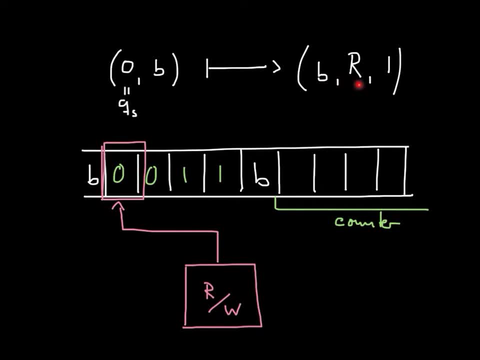 So we write the blank symbol again, go right and go to state 1.. So after executing this instruction, our Turing machine would be in state 1 and would be pointed one cell to the right of the initial cell, which is this cell. 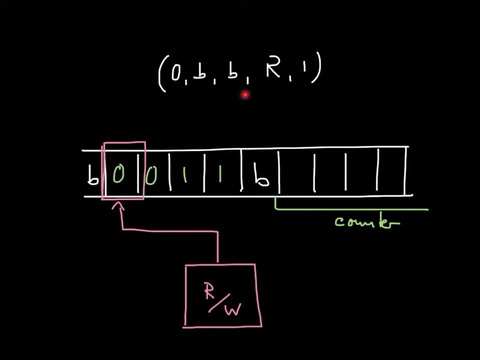 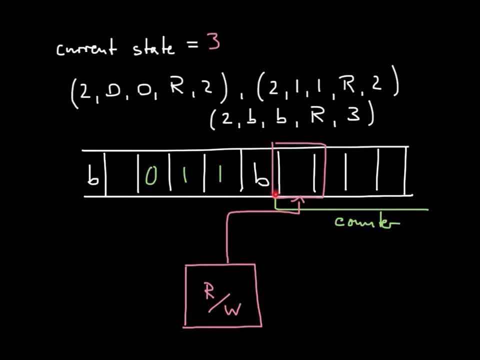 be on this cell and be in state 3.. So now we have reached our counter, and if we get there for the first time, of course there will be a blank in here and we just have to write a 1 to put in the first bit. 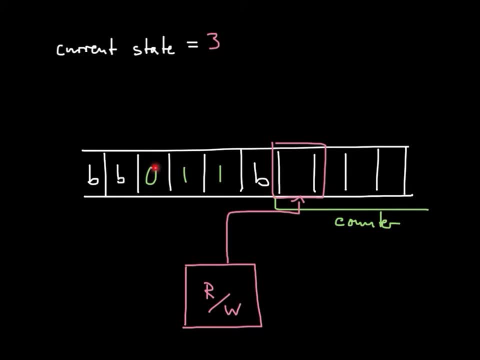 for our counter. If we have read multiple zeros of the input already, then there will be already a few 1s here and we just have to now first go to the end of the counter, so to the first blank to the right of the counter to add a 1 there. 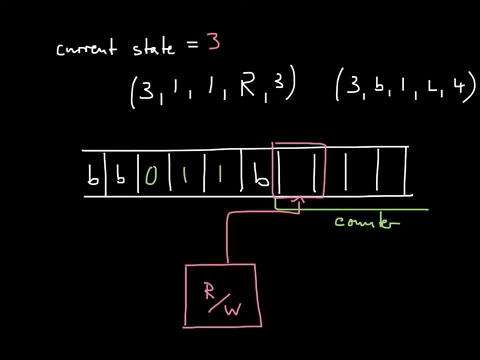 So this increase of the counter is accomplished by those two instructions here. So the first one just says: well, as long as I'm not at the right end of the counter, just go right. As long as I read 1s, The 1s. 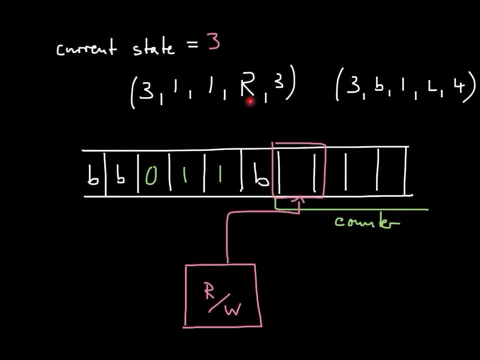 The 1s symbolize the counting bits right, Go right and stay in state 3.. However, when I reach a blank, replace this blank by a 1.. That means we increase our counter by 1, and then we can go left and go into state 4,, where 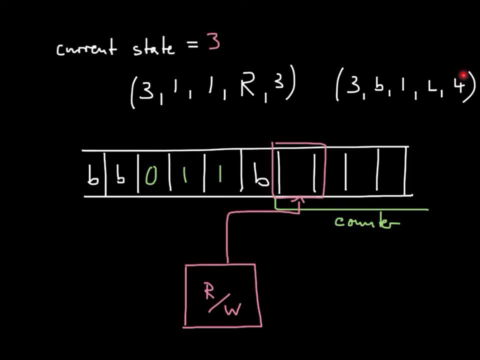 state 4 now means go all the way back and do the same thing again, So running our program here. we would put a 1 here, because we're already at the right end of the counter. It was 0. So far, right. 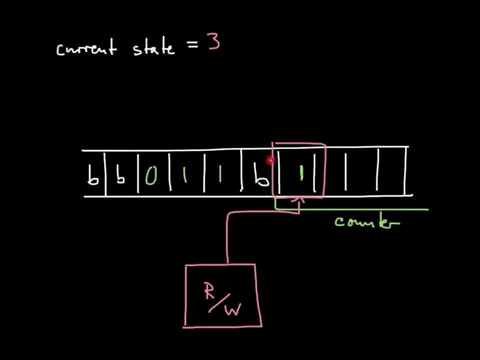 We put a 1 here and now we would go 1 to the left and enter state 4.. The next thing we would do is now move all the way to the left again until we hit the first blank to the left of the input. 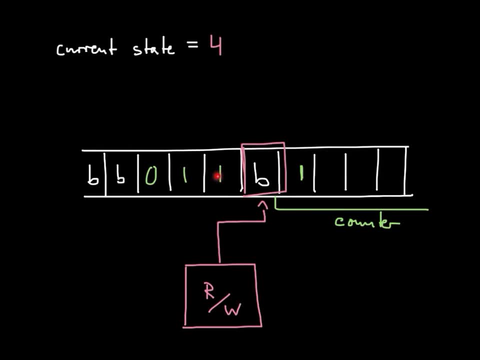 Remember that we deleted the first bit already. So by reading through the input we will successively put more blanks here, so we don't need to read it all over again. We just need to read the remaining bits here. So we would now go back here using a similar routine that we did use before to go all the 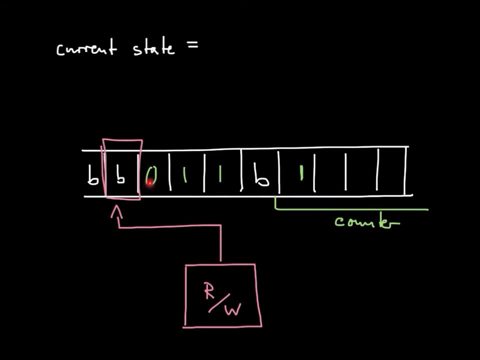 way to the right of the input and then start over again. So if we go 1 to the right, read a 0, we go all the way over here, go to the right of the counter, put a 1 there and then go back to the left of the input. of course this 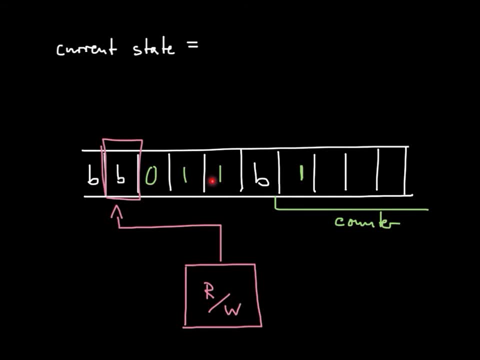 0 here will then be replaced by a blank, and so on. So eventually we will have read all the 0s, replaced them by blanks, and have a counter here that represents the number of 0s we have read. Well, now we do the same thing. 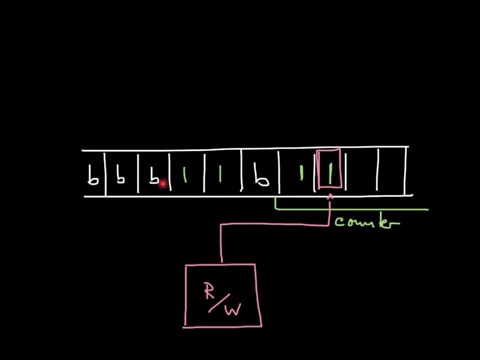 We go back to the left of the remaining input and then in the next stage we see: oh, we're not reading 0 anymore, But we're reading a 1.. So in that case we have to go now and start deleting bits from our counter. 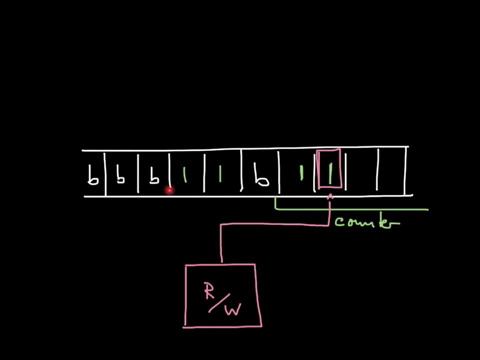 So if we read a 1 here instead of a 0 after going back all the way to the left of the remaining input, well, we go into delete mode. We go seek the first blank here, then seek the end of the counter. replace the last bit. 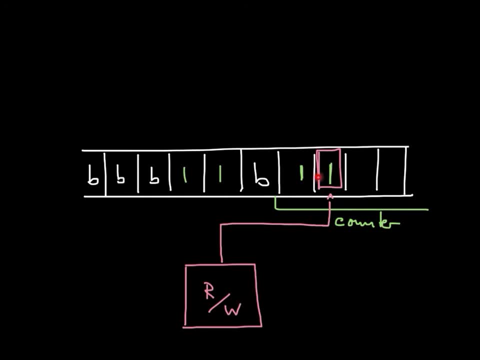 of the counter by a blank. So after we've done that, we go back, go to the next remaining bit of the input, go back again, go to the end of the counter, replace it- the 1 there- by blank, and then go back. 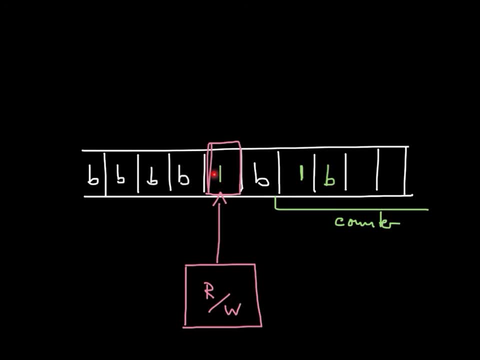 again till we eventually don't find a 1 anymore. So that's it. Thanks for watching Bye. And if, in the end, our counter is all the way reduced back to all blanks, so 0 again, well then, we accept. 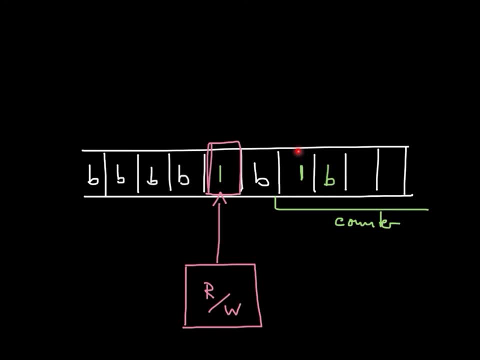 Of course, in this whole procedure there's a lot of things and details we have to pay attention to. For example, what if we read a 1 directly instead of a 0 first? Or if we don't read anything, If we have an m?